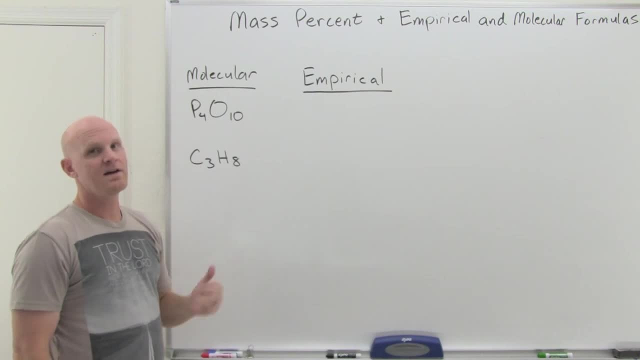 a single molecule of tetraphosphorus decoxide, there are four phosphorus atoms and 10 oxygen atoms. Now the empirical differs from that, And I say differs because it doesn't always differ, it turns out. But in this case it differs because the empirical is going to be the most reduced. 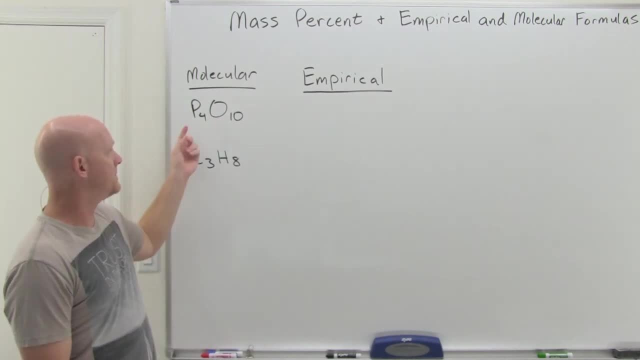 integer or whole number ratio, however you want to look at it, between the atoms. So a 4 to 10 ratio, those are both divisible by 2. And so we can reduce that down to a 2 to 5 ratio And that 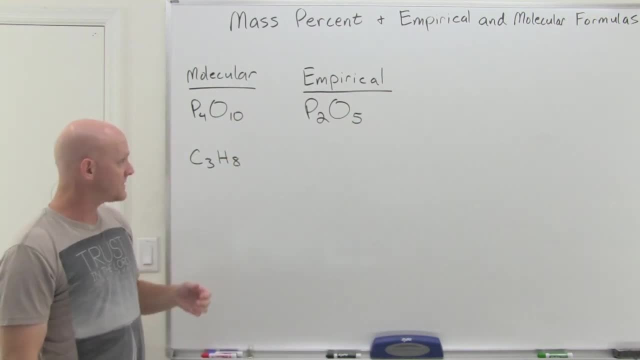 would be the empirical formula instead. Now, for a lot of compounds, it turns out that your molecular and your empirical will end up being one in the same. If your molecular formula happens to have the lowest integer ratio, well, that's going to be your empirical as well. That's the case here. 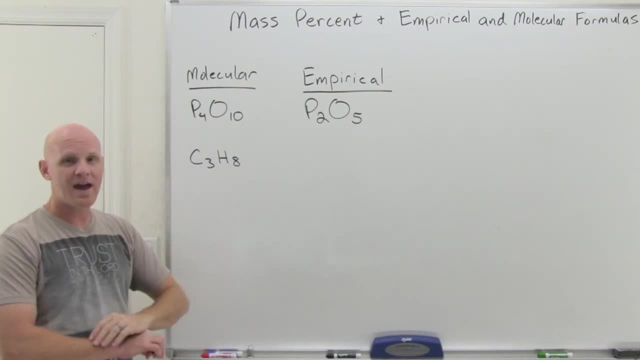 with propane at C3H8.. That 3 to 8 ratio can't be reduced any further, And so in this case the empirical formula would also be C3H8. And this is not uncommon to see both- you know, molecular and empirical being the same for. 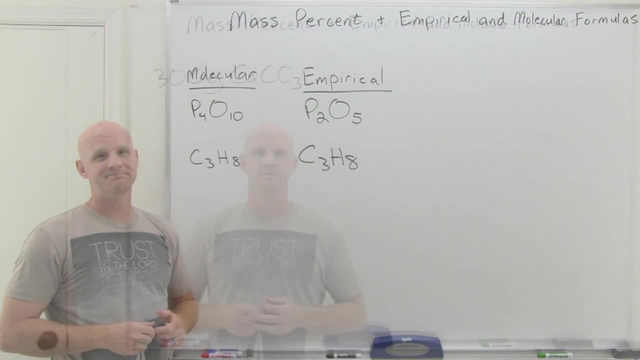 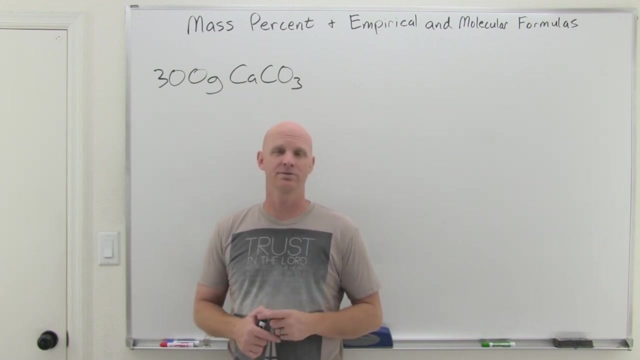 compounds, So could see examples of either of these types. So now we're going to take a look at mass percents And we're going to eventually see how the mass percent can be related to both the empirical and molecular formulas. And so we'll start with just plain old mass percents here, And 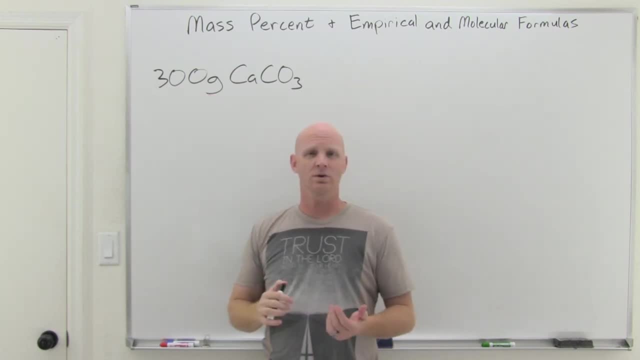 so we're going to take that 300 gram sample of calcium carbonate we dealt with in the last lesson And we're going to explore it And we're going to find the percentage of carbon in the sample and the percentage of oxygen in the sample And so in this case we've got 300. 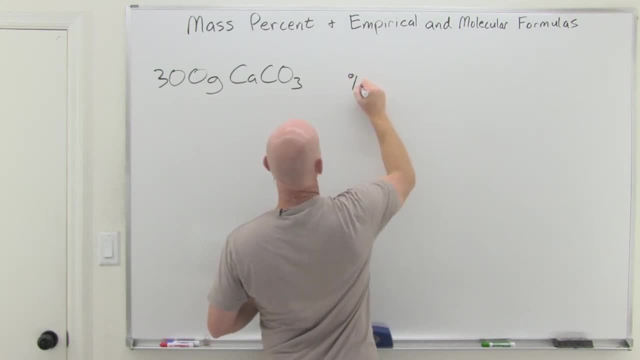 grams. And you might be like, okay, well, if we want that percent carbon, well, percent carbon is going to equal the grams of carbon over the total mass times 100. And so we might look at our sample and be like, well, it's got 300 grams, And that is true, But we have to figure out how many of those. 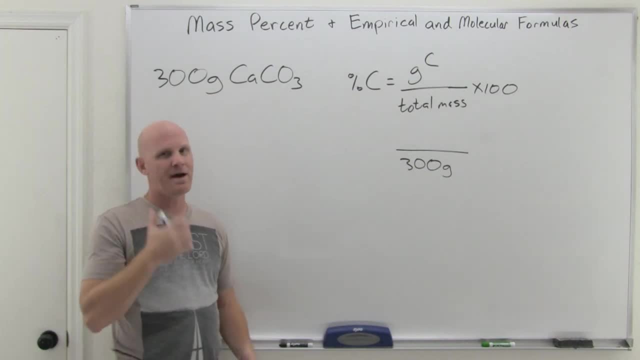 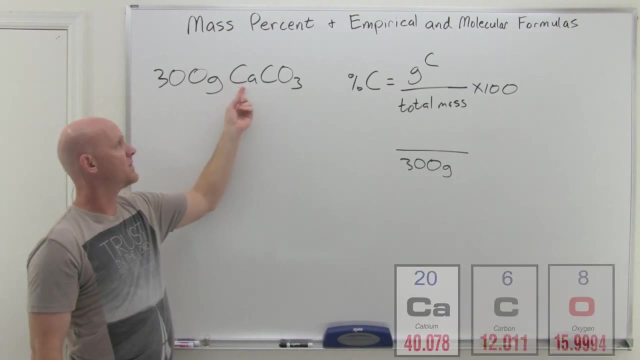 300 grams are carbon And that's going to be a little bit problematic. So in this case we've got nice numbers. So you might recall that the molar mass for calcium carbonate is 100. So calcium is around 40. Carbon is around 12.. Each of the auctions are 16. each Three times 16. 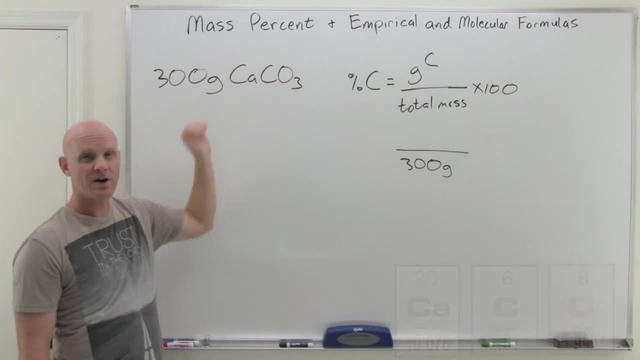 is 48 plus 12 is 60, plus 40 is 100. So a molar mass of 100 grams per mole, which makes this convenient, And we can see that 300 grams then would be three moles And every mole has one. 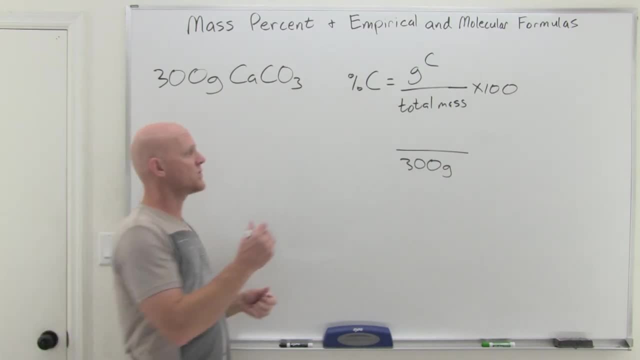 mole of carbon. So three moles would have 36 grams of carbon, And we could write that all out. So, and then times 100, except I don't want to do this. That was more work than I wanted to accomplish, because it turns out that these mass percents are an intensive property, which means it doesn't 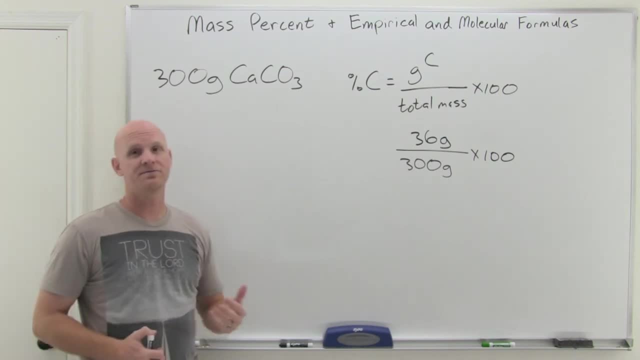 depend on what size of sample you have. Whether I had 300 grams or five grams or a million grams, it doesn't matter, The mass percents were going to work out exactly the same way, And so if you actually know the formula of your compound, it's actually quite often convenient So to not use the actual 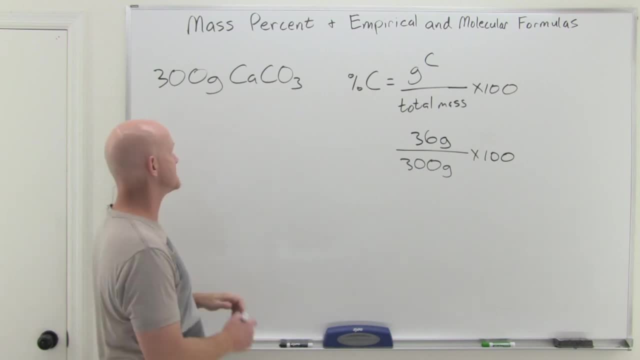 size of sample that you have, but to choose a one mole sample size. And so, once again, if we did 100 grams, it would only weigh 100 grams. And the key is is that in one mole of calcium carbonate, I can really easily see that there's only one mole of carbon, one mole of calcium, three moles of. 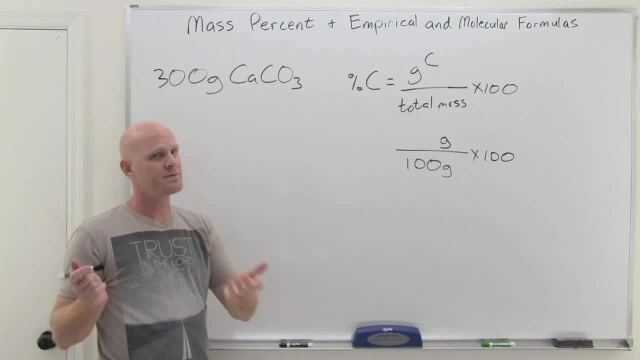 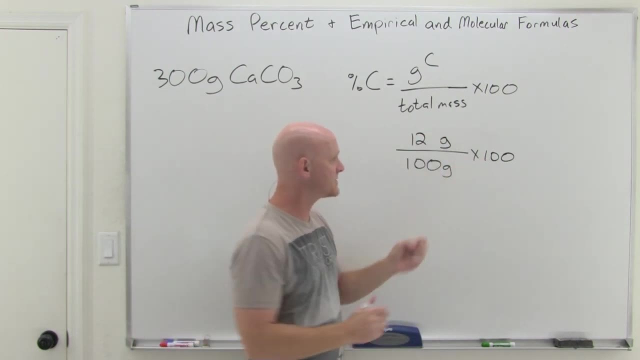 oxygen, And so in this case, for carbon, there's only one mole of carbon, and one mole of carbon right off the periodic table weighs 12 grams, And so here makes doing percentages here real easy as well. 12 over a hundred times a hundred is going to get us 12%, And again had we done. 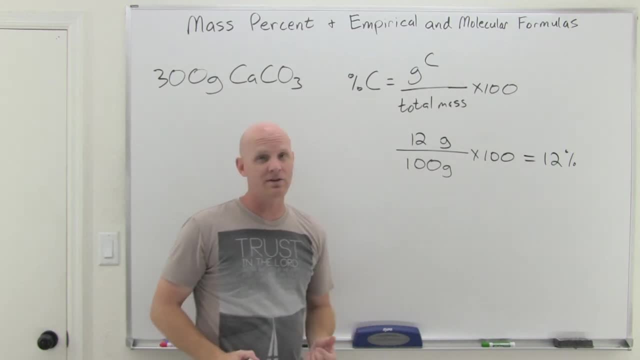 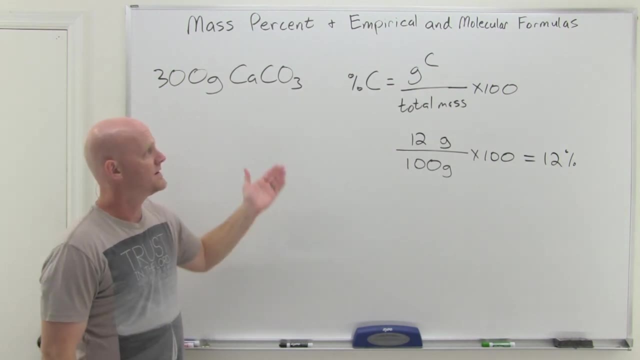 36 grams out of 300 grams times a hundred, we would have got the same answer. It just would have been more work. We had to figure out how many moles of this we had and then how many total moles of carbon were in that sample, And it's just more work, Whereas, again, if you know the formula, 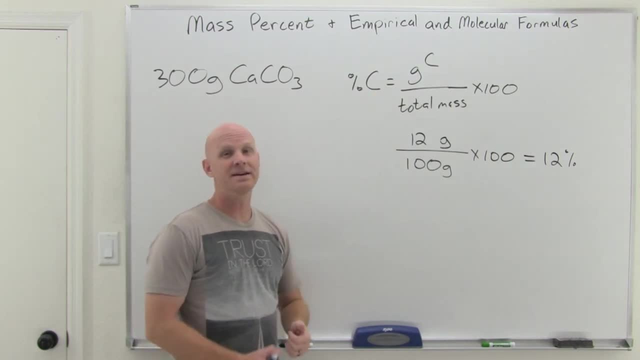 a one mole sample size is really convenient And with mass percent being an intensive property, we can choose any sample size we want. Okay, So now we want to find that percent oxygen as well, And in this case same general property, So grams of oxygen over total mass. 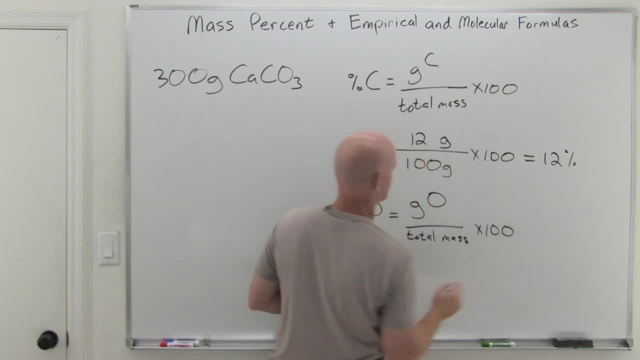 times a hundred. but this time we'll take advantage of the fact that we're going to use that one mole sample size, And so that total mass is once again going to be a hundred grams for calcium carbonate. So one mole sample, But in this case in one mole of calcium carbonate. 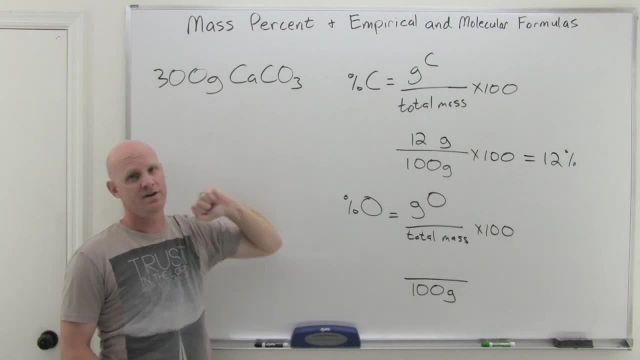 there's not just one mole, like there was with carbon. there's three moles of oxygen, And if each mole of oxygen weighs 16 grams, then three moles is going to weigh a total of 48 grams, And then times a hundred. 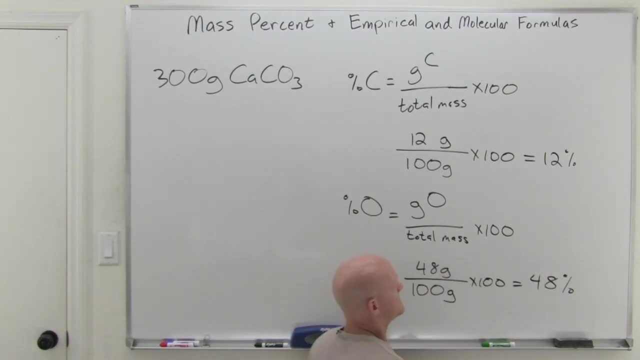 and we get 48%. So in this case, 12% carbon, 48% oxygen and we could deduce that the rest is calcium. So it had to be a total of 40% calcium, which we could calculate it the same way or just. 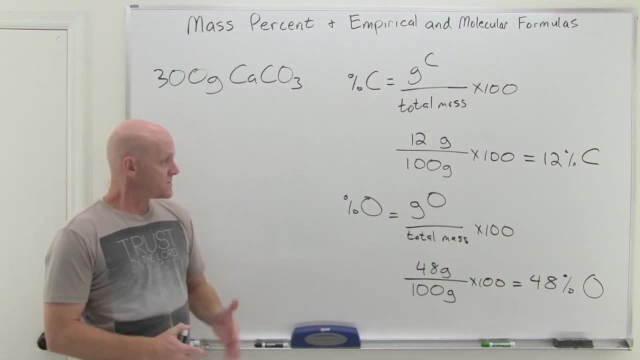 subtracted, these total from a hundred. Cool. So this is how you take an empirical or molecular formula, or chemical formula, as the case may be, and turn it into mass percents. But you can also do the exact opposite. You can take mass percents and turn them into an empirical formula. It's a much greater pain in the 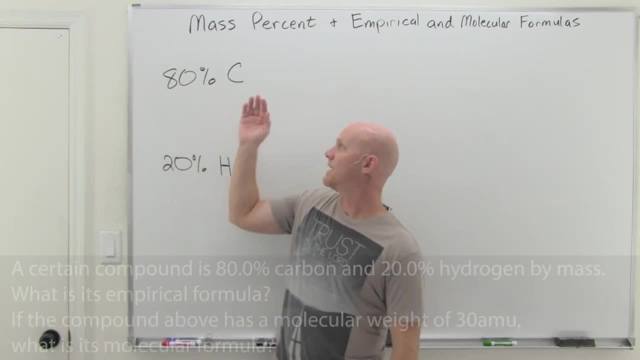 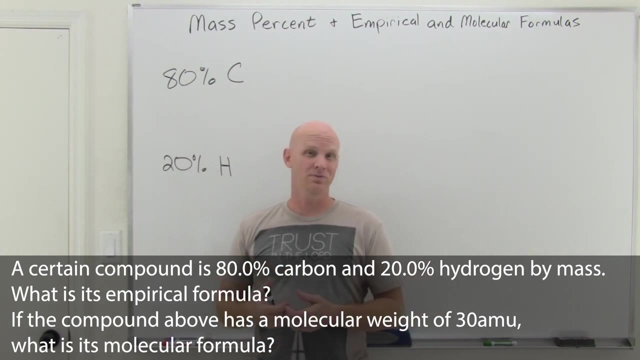 butt, as we're about to see. So in the next question we've got a compound is given as being 80% carbon by mass and 20% hydrogen by mass, And the question is: what is its empirical formula? That's the. 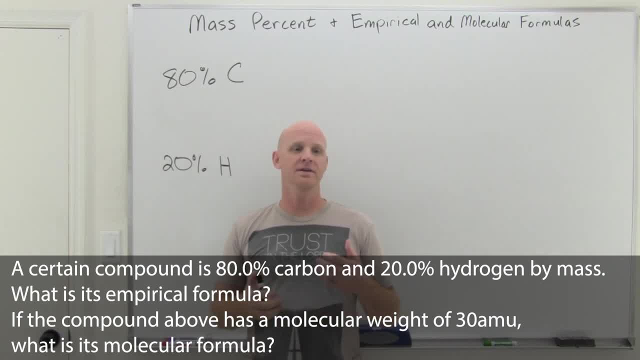 first question: After figuring out its empirical formula, we're then told that the molecular weight of this compound is 30 AMUs, or we could have been told that the molar mass was 30 grams per mole- Same diff. And then we're asked to find further the molecular formula. 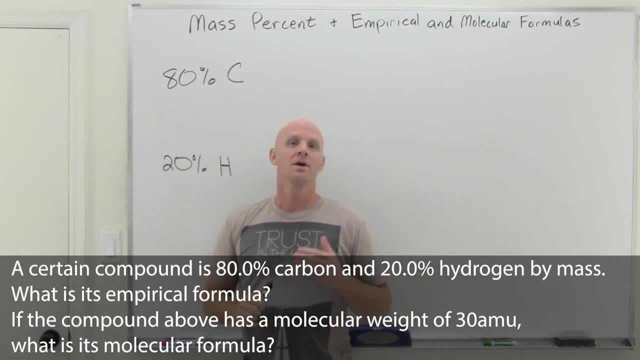 Now it turns out, from mass percents alone you can get the empirical formula. So on top of that, though, you need a molecular weight or molar mass to then take that empirical formula and turn it into a molecular formula, as we'll then be tasked with here. So all right. so how do we go ahead? 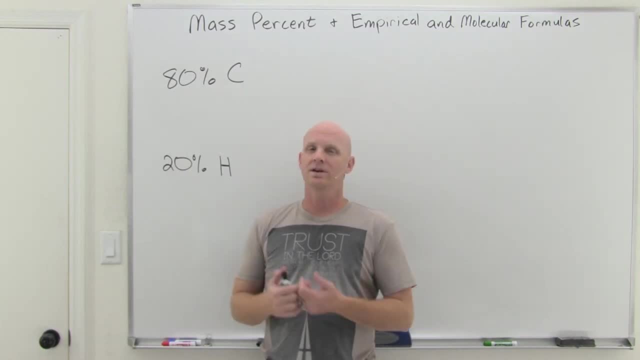 and do this. Well, how do we turn a mass percent into an empirical formula? Well, again, when we took an empirical formula and turned it into a mass percent, we figured out. you know, mass percents are intensive, We can use any sample size we want. And so we chose to use one mole. Well, I can't use. 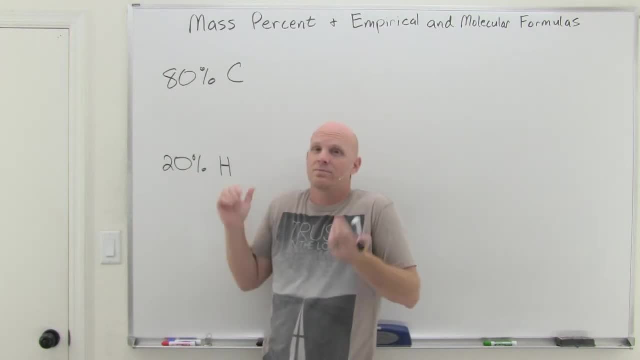 one mole here because we don't know the formula. If I don't know the formula, then how can I ever predict how much one mole would weigh? So but there is still a convenient sample size to use. So, regardless of how much of this particular substance we may or may not have, it's convenient. 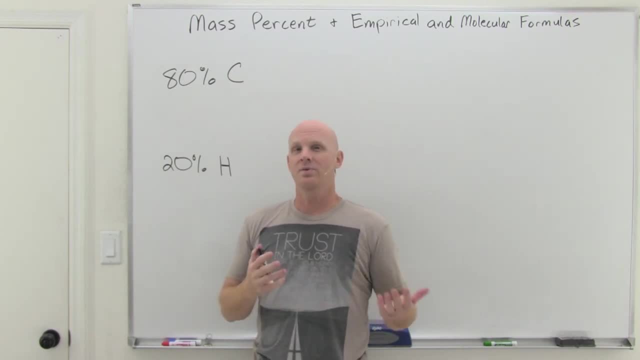 now with mass percents to just say, well, what if I had a hundred grams? And the reason that's convenient is it takes a little of the math out. So because 80% of a hundred grams is 80 grams, That's easy, I can do that in my head. Whereas had I chose like, well, I'm going to choose 217.436. 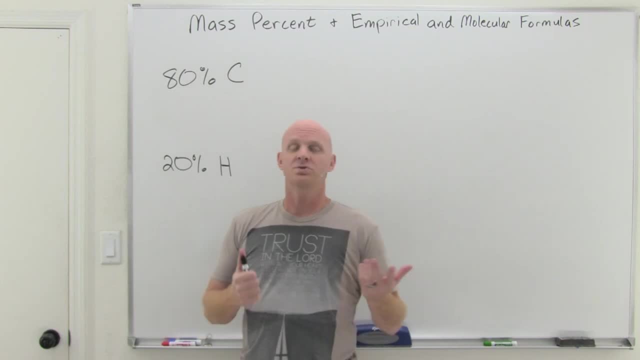 grams. Well, 80% of that. now I got to pull out my calculator and stuff, So so we're going to save a little time by just assuming a 100-gram mass per cent. So we're going to save a little time by. 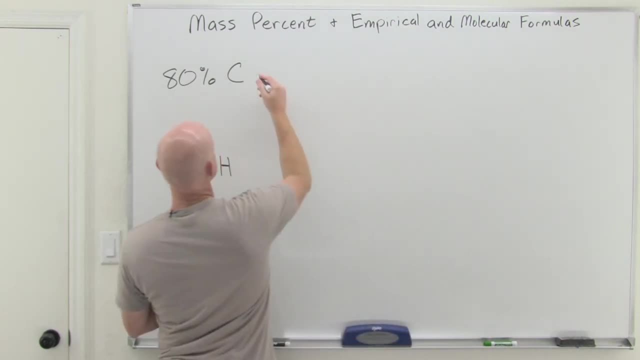 just assuming a 100-gram mass per cent. So we're going to save a little time by just assuming a 100-gram sample size. And so in this case, this 80% carbon is going to turn into 80 grams of carbon. 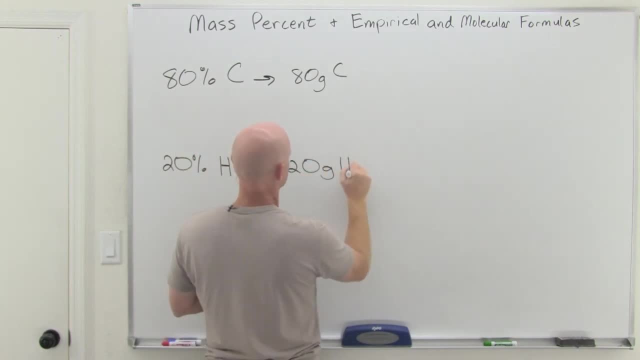 and this 20% hydrogen is going to turn into 20 grams of hydrogen. Now, if we take a look at our formula, we want to end up with? we want to end up with something like C, X, H, Y. 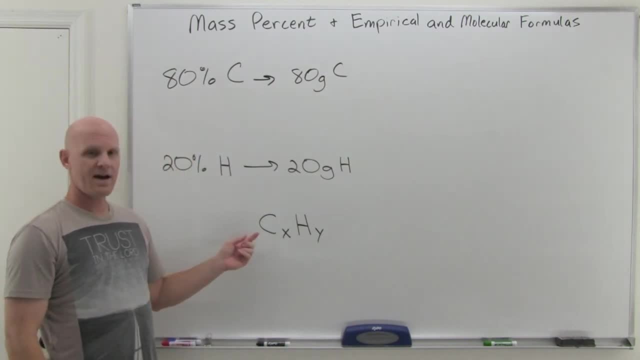 where X and Y are going to be an integer ratio of the number of atoms, or moles of carbon to hydrogen, And in this case then it is a mole to mole ratio is one way to look at it, or atom to atom ratio, So, but I'm going to look at it as a mole to mole ratio, not a gram to gram. 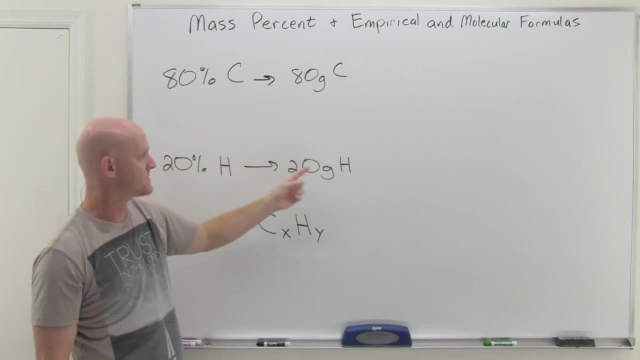 ratio, And so in this case, you might look at this and be like: oh, 80 grams for every 20 grams of hydrogen. Well, that's easy, Chad, That's going to be four times as much carbon as hydrogen. And 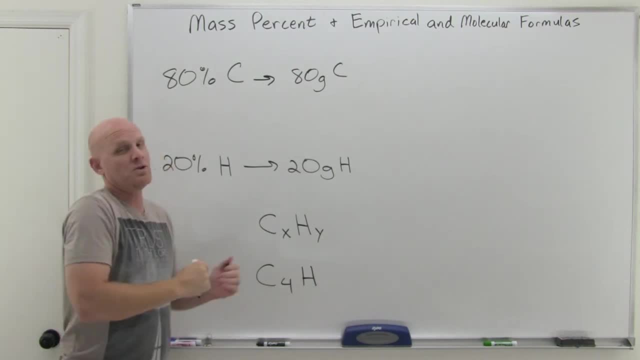 C4H1 is the same thing as just C4H, And I didn't even have to pull up my calculator. Well, this is wrong, right? Because this four to one ratio is not a ratio of grams. Again, it would be a ratio. 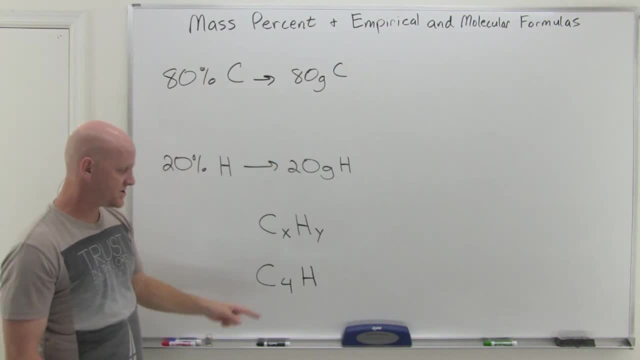 of moles, and 80 grams to four to 20 grams. that four to one gram ratio is not what should be represented here. This is totally wrong. So I'm going to look at it as a mole to mole ratio, not a. 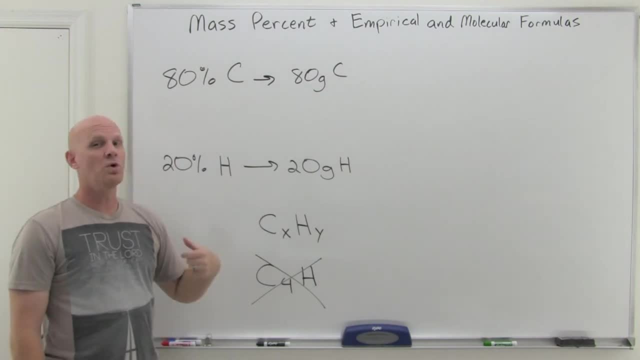 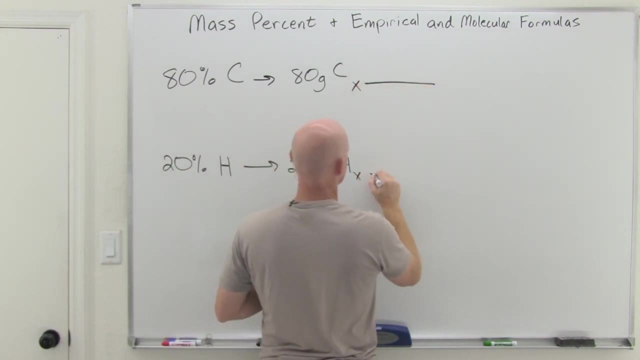 totally wrong, And so what we've got to do to figure out a mole to mole ratio is then have moles, and these are grams. So the first thing we'll do here is convert to moles. And how do you convert grams to moles? Always through the molar mass. We'll put grams of carbon on bottom moles of 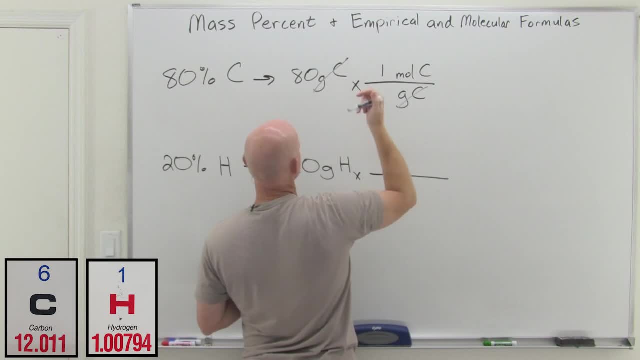 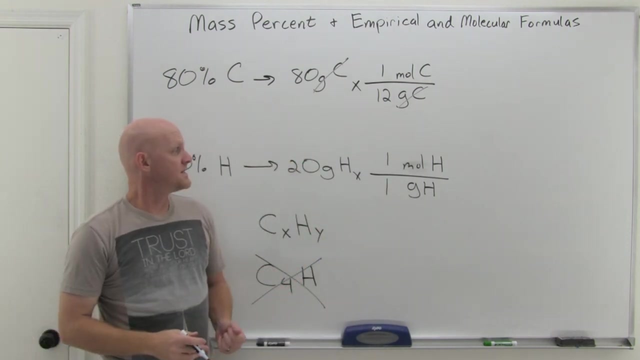 carbon on top. That way these cancel. And the molar mass here one mole, if you look up on the periodic table, weighs 12 grams. in the case of carbon, Same thing here: grams of hydrogen on bottom and moles of hydrogen on top. So, and in this case, one mole, one gram, And in this case, 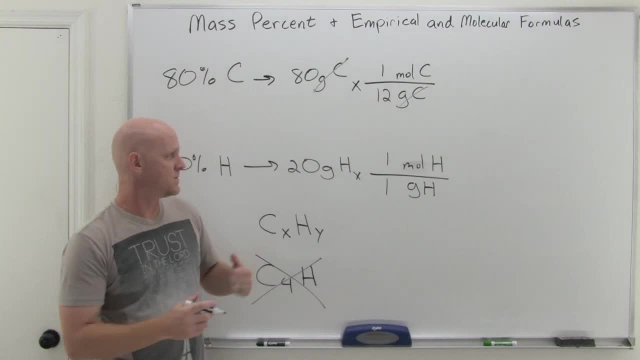 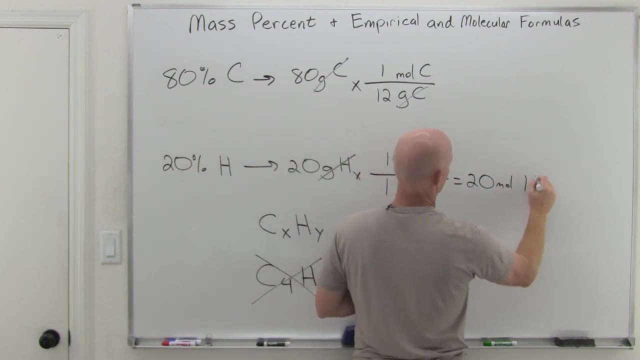 then we're going to move on and turn these into moles, So grams of hydrogen here cancel as well. And so this one's easy: 20 times one over one is just 20 moles of H, And then 80 divided by 12,. 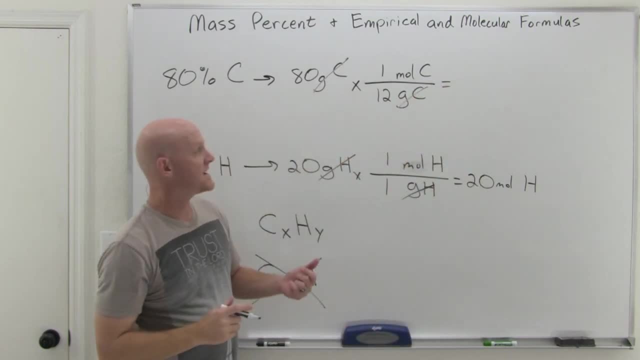 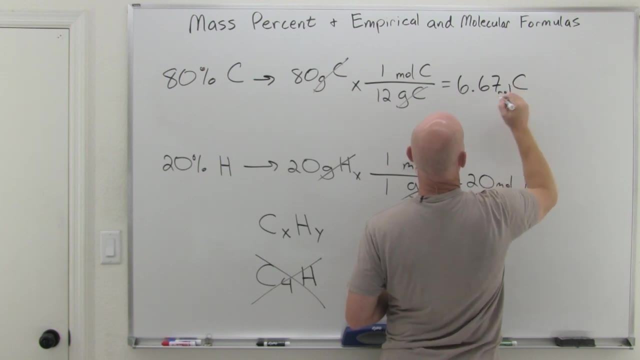 not so easy to do. in your head. It's possible, But it's going to come out, in this case, to 6, 2, 3rds or so. what I'll round it to So 6.67 moles of carbon, And so, in this case, that's now a. 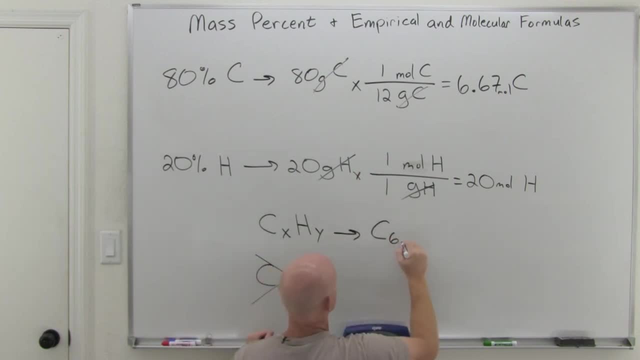 mole to mole ratio, And so we can see that this is C 6.67,, H 20, and voila. life is good, right So? but there's a problem, right? Because this is supposed to be an integer ratio and 6.67 is not. 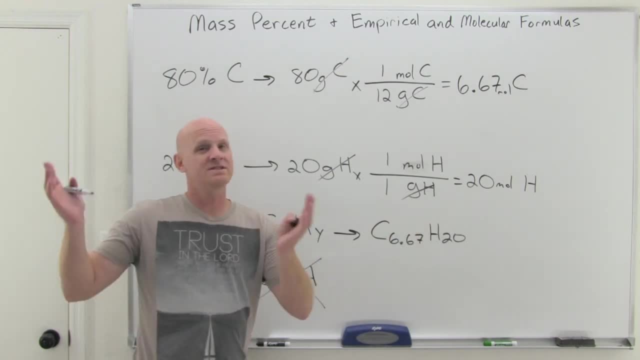 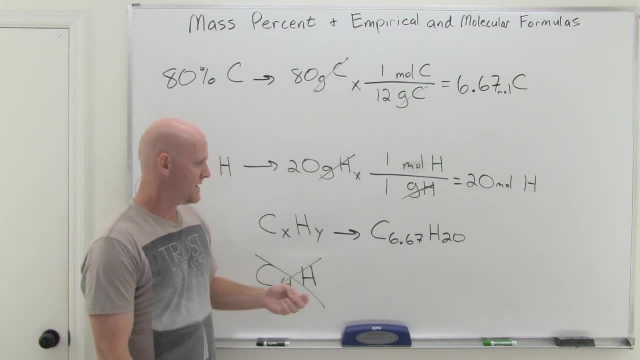 If it doesn't come out to integers, you have to get a little creative on how to get it there And, in this case, one way to for sure, when, again, we have to keep this ratio, exactly the same fundamental ratio, just with integers instead, And so what we typically do here is we divide both of. 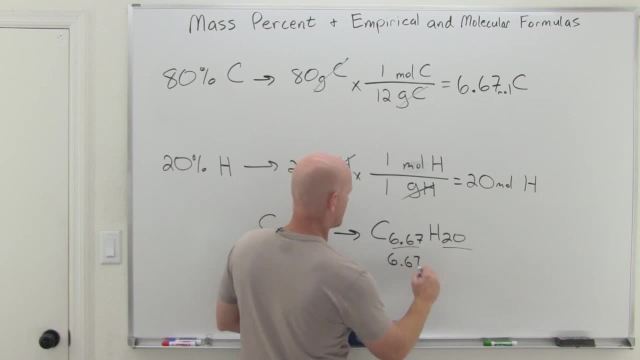 these numbers by a common factor. Whichever of the two numbers is lower is that common factor? because this guarantees that one of the numbers is going to come out to be an integer. It's going to come out to be a one, And so in this case it turns out this comes out to C. 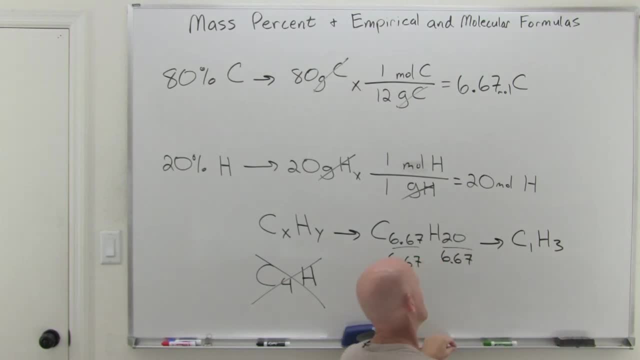 one H three. 20 divided by 6.67 is almost exactly three, And as long as this comes out to almost exactly a whole number, well then you're good, And we have C one, H three, which is the same thing as C H three, And that is our empirical formula. Now, this doesn't always come out to 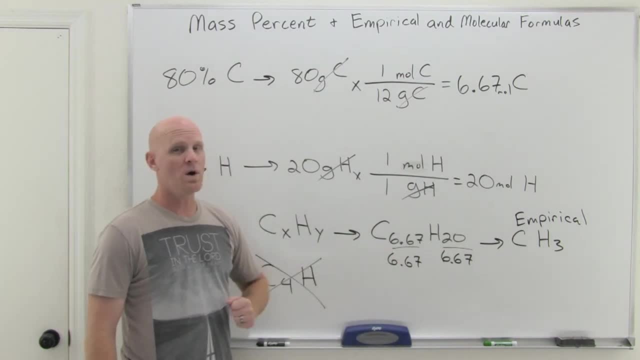 two whole numbers right off the bat. Again, you're guaranteed to get one of them as a whole number of the whole number of one. But what if you know the other one doesn't actually come out really close to a whole number? Well, don't round it, Don't round up, Don't round down. So 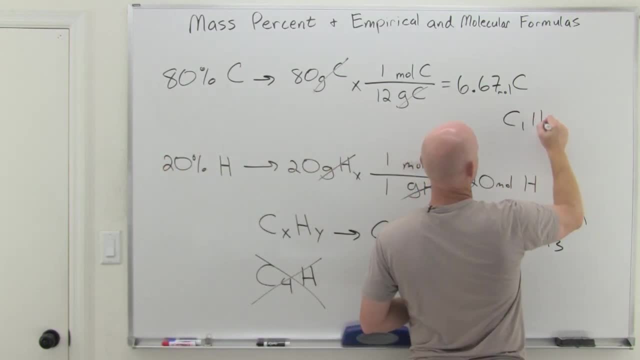 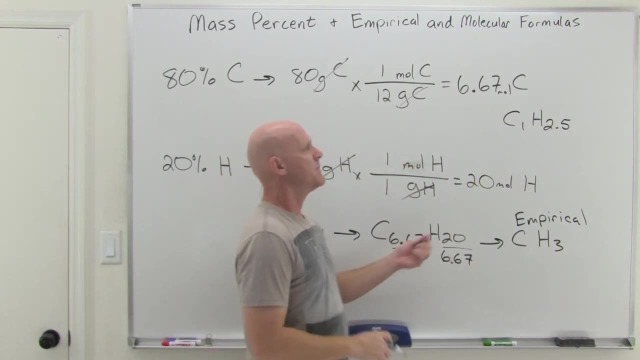 because what if this had been like you know, C, one, H, two point five? You wouldn't be like, well, I'll just round it up to three. You don't want to do that, because then you're actually fundamentally changing that ratio. But what you want to realize? that you've got a half here And 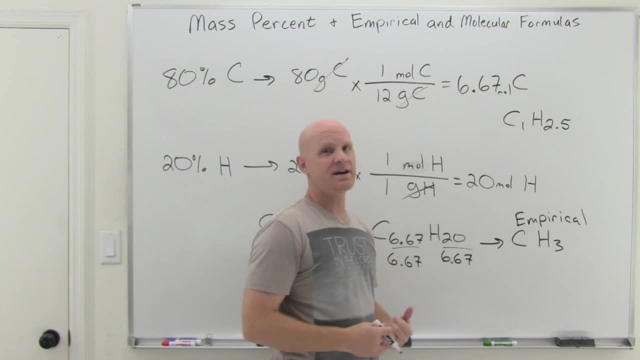 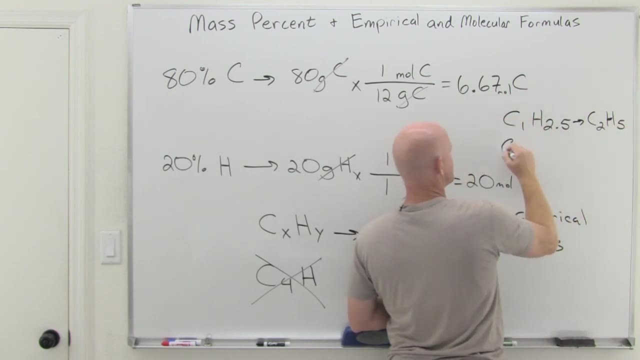 when you've got a half. so you need to double it to get up to being integers. And so if you double the whole thing, that would get you to C two, H five. Or what if this had been C one, H one point. 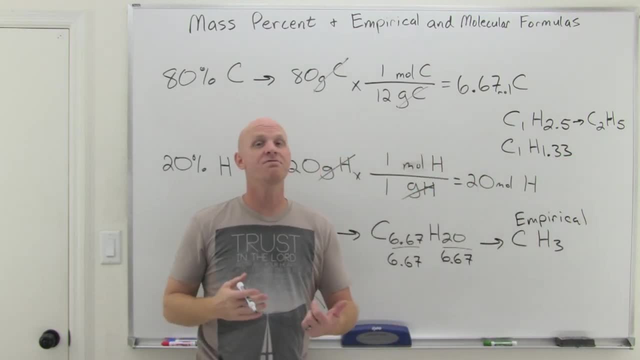 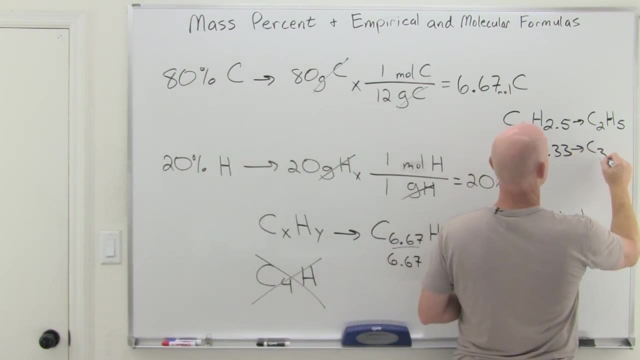 three, three. Well, you've got to realize that point three, three is a third. And how do you get rid of thirds? Well, you multiply by three. And if we multiply this whole ratio by three, we then would have got C, three, H, four. Cool, But in our case it just happened that it came. 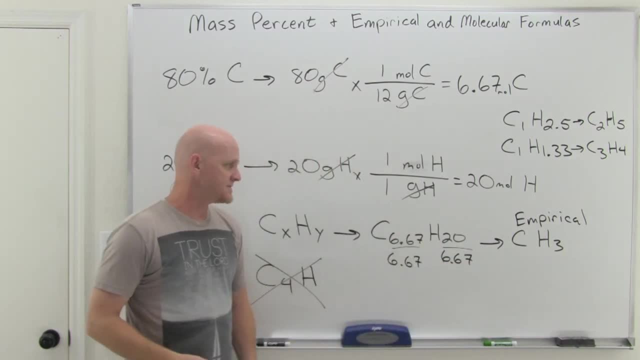 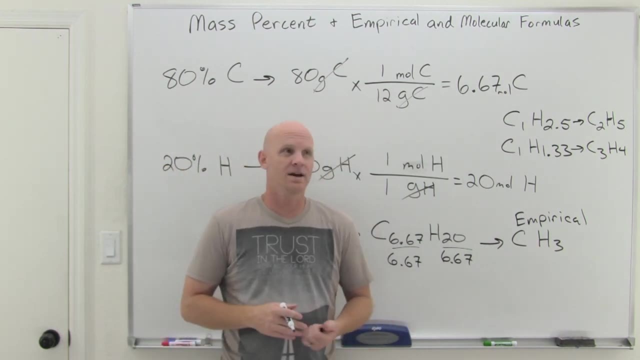 out to two whole numbers, a one to three ratio, exactly. So life is good. And that's our empirical formula. Now the second question we're asked is: what's the molecular formula? Well, if we weren't given any more data, we just say: I don't know, Maybe it's that, Maybe it's C, two H. 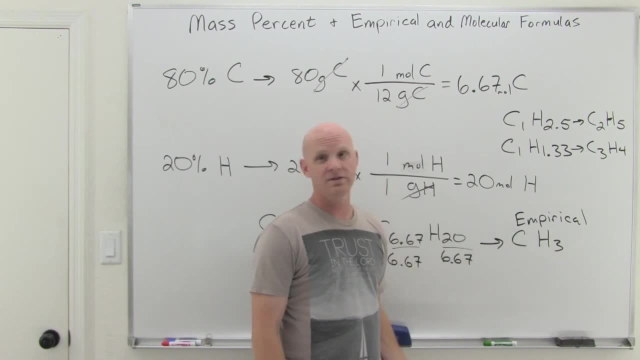 six C three H, nine C, one thousand, H three thousand C one million, H three million. There's an infinite number of one to three ratios that are possible, And so one other piece of information has to be given to you, and that is the molecular weight or molar mass. And so 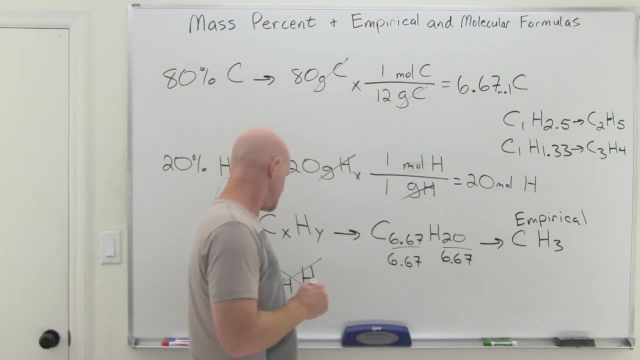 in this case, we're told that it weighs 30 AMUs. Well, if we take a look at CH, three for a second, So carbon weighs 12.. Each of the three hydrons weighs one each, for a total of three more. So 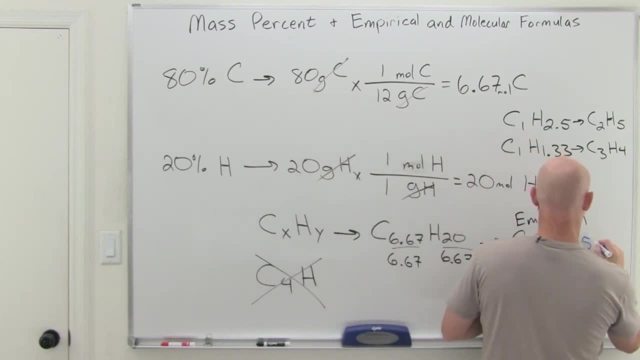 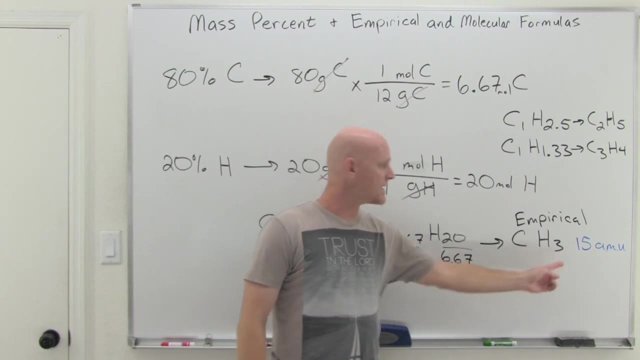 12 plus three is 15.. And one thing you have to realize is that when you start doing multiples, if you double the whole formula, that also doubles the weight. If you triple the whole formula, it would also triple the weight. And so whatever your molecular weight is going to be in this case, 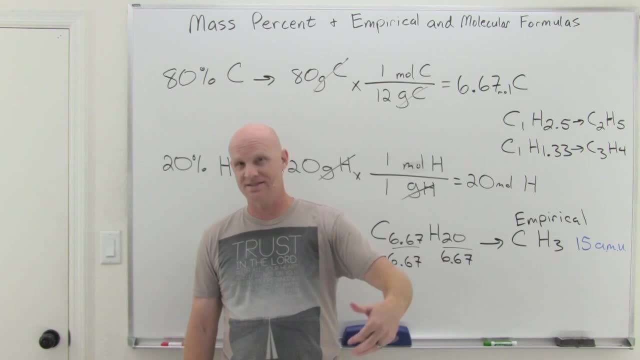 it has to be a multiple of 15.. It's got to be 15,, 30,, 45,, 60,, 75,, et cetera, And it's going to be one of those. And in this case we're told actually that it is 30 AMUs. And so the question: 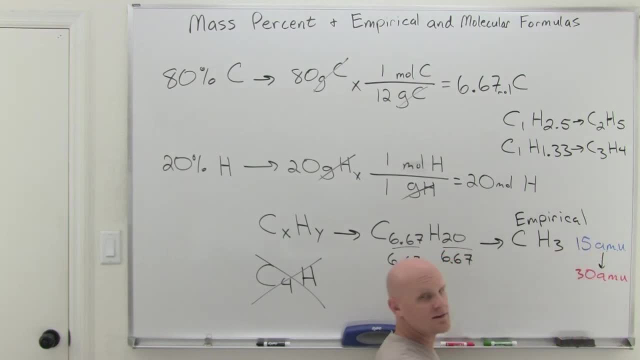 is then? well, how do I get from 15 to 30?? Well, I've got to double the weight. And if I'm doubling the weight, that means I'm doubling the formula here as well. And so there indeed is our molecular formula C2H6.. Had we been given a molecular weight of 45,. 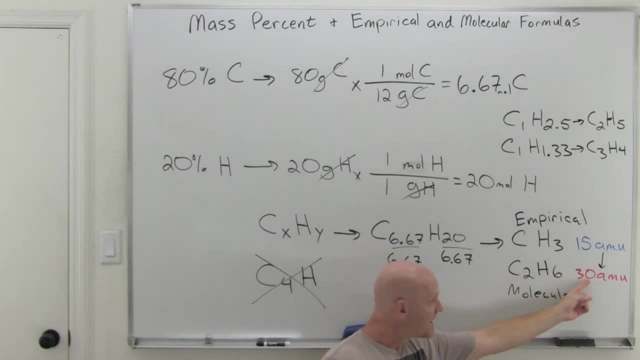 then it would have been C3H9.. Had it been, you know, 75,, then we would have multiplied by five and been C5H15 or something like that. So we had to have that fundamental one to three ratio. We. 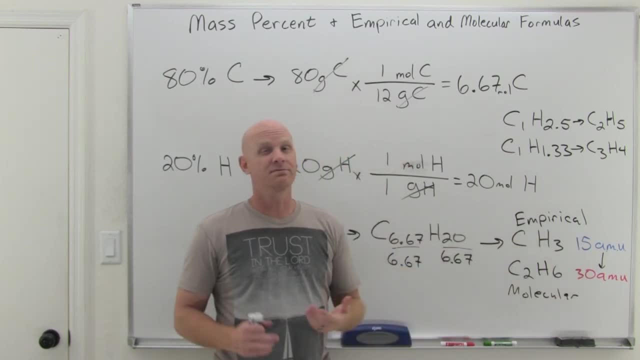 just need to know what multiplier, what multiple of the formula to give, based on the provided molecular weight. If you found this lesson helpful, please give it a thumbs up, And if you want to learn more about this lesson as well, a like and a share go a long way to making sure other students get to see this.